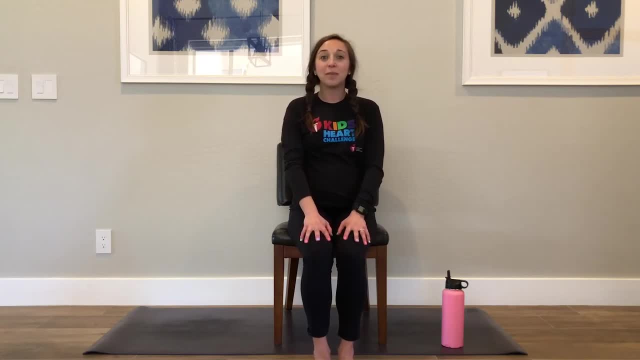 hands right there on our legs and we're going to begin by taking a deep breath in, So breathing in and rolling our shoulders up towards our ears and down our backs. All right, let's do that one more time: Breathe in shoulders up towards your ears, Breathe out down towards your back. 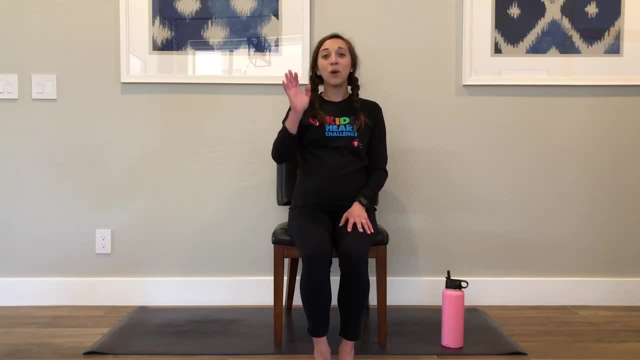 Great job, everyone. Next, we are going to take one of our hands and place that hand on the side of your chair. Take the other hand and place it on the outside of your leg and we are going to do a slight tilt. So rotate your body, your spine, Make sure you're still standing up straight and take your eyes. 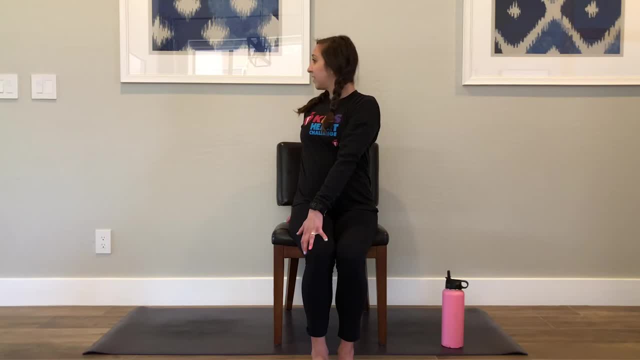 towards your back shoulder. You should feel this stretch in your body and your spine. All right, bring it right back around to the front and we're going to switch that out. Go ahead and take that opposite hand, place it on the outside of that chair and your other hand to the outside of your leg. Begin to twist your body. 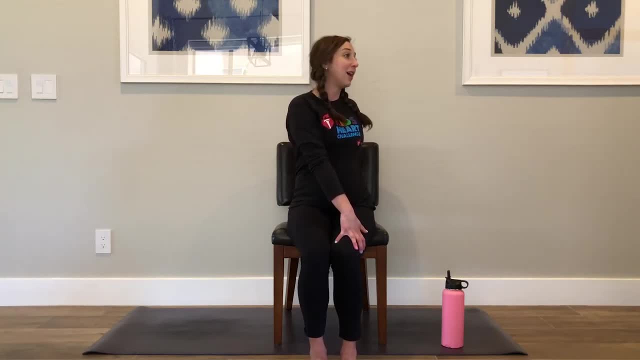 and take your focus or your eyes to your back shoulder. Great job. Next, we are going to take our leg and put it up on our other leg. Okay, so this should create a v-shape. Rather than pointing your toe like this, we want to flex it. 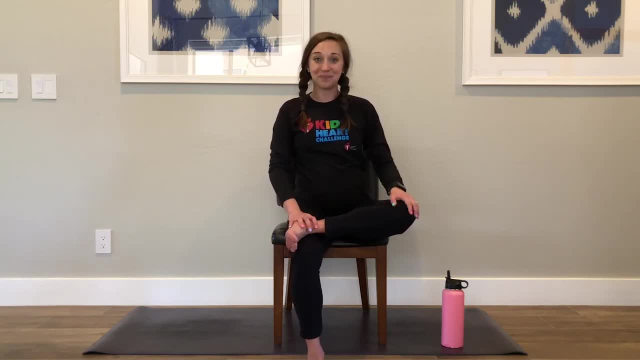 so that it is straight. This will help protect your knee. All right, sit up straight, Make sure your foot on the ground is stable and if you want a further stretch, you can begin to lean forward ever so slightly to help feel that stretch on the outside of your leg. You should never feel pain. 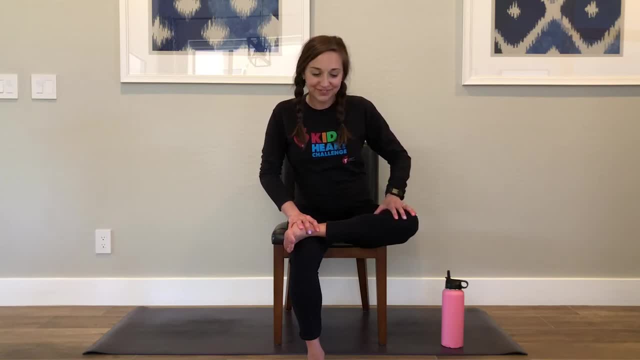 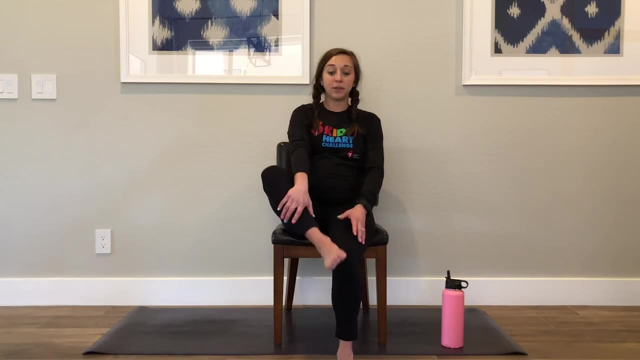 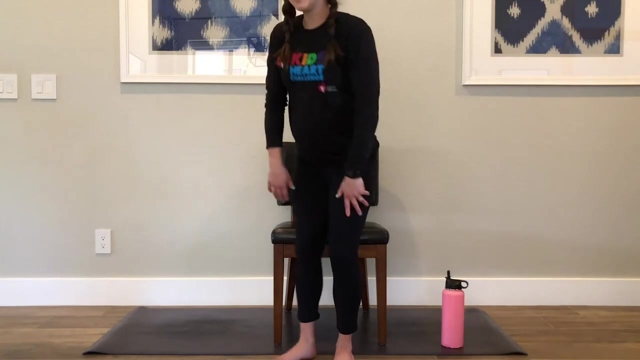 just a nice stretch. Go ahead and switch that out. Place that foot down on the ground, bring that other foot up towards your thigh Again. remember to flex your foot back towards you and lean forward. Great job, everyone. Next we are going to stand up. Next we are going to do the comprehensive. 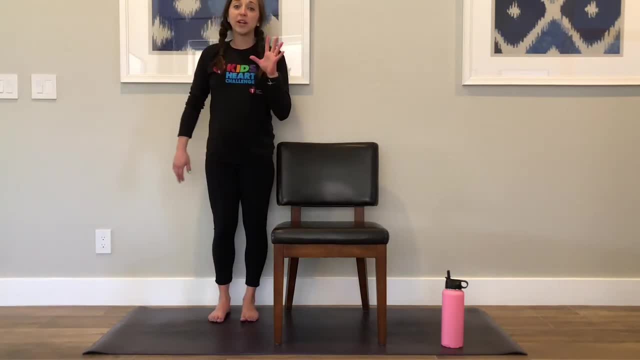 bend our chair, okay. so once we're next to our chair, we're going to take that hand and place it on the on the chair for support. we're going to put the foot closest to the chair, planted firmly on the ground, and our outside leg is going to come up into a kickstand like this now with our hand on. 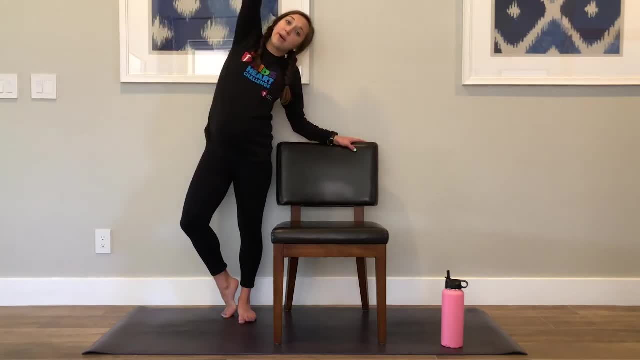 that chair. we're going to take our outside hand and we are going to rainbow over the chair. make sure you're holding that chair for support. you should feel this stretch on the outside of your body right here. go ahead and lean into it all. right now let's come back up and switch to the 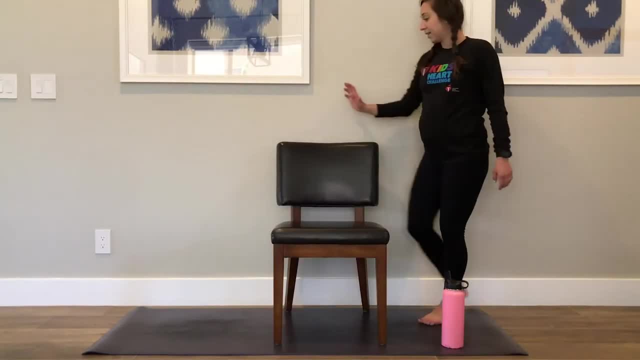 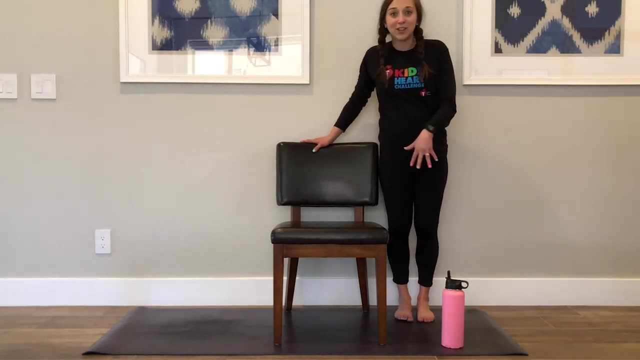 other side. place that hand on your chair again. the foot that's closest to the chair we're going to plant firmly into the ground. the outside leg is going to come up into a kickstand and we're going to lay, we're going to prop up as a kickstand, hold on to that chair and rainbow over the chair on the. 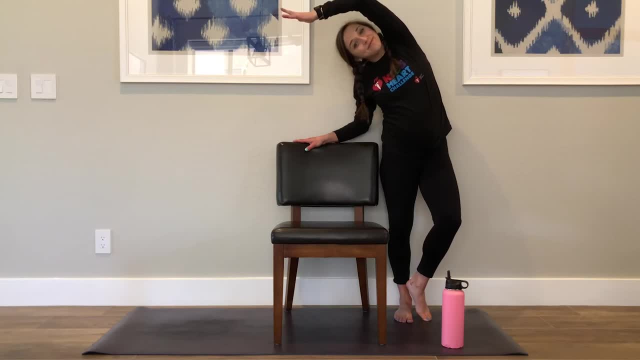 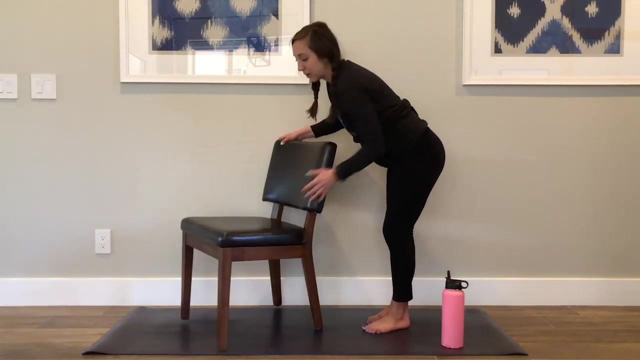 opposite side, bring it back up. oh, that should feel so good. okay now. what we're going to do next is come around to the back of our chair. okay, so I'm just going to turn mine and on the back of our chair. what we're going to do is we're going to place our hand on the outside leg and we're going. 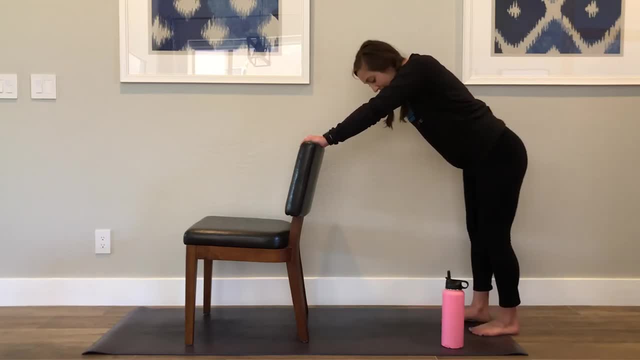 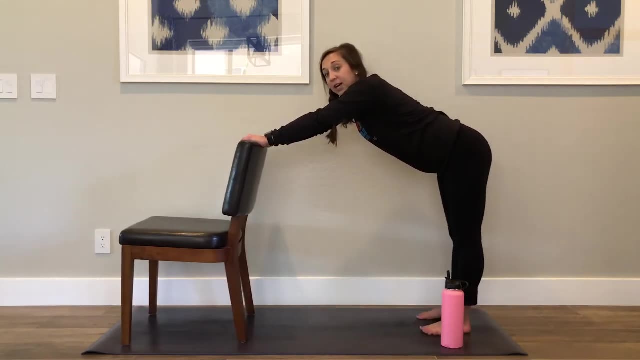 to place our hands firmly on that chair. we're going to take a couple steps back so that knee okay, so a couple steps back from your chair, and so we are in this position. now what we're going to do is we're going to bend slightly, bend our knees, and we're going to drop our head and our shoulders. 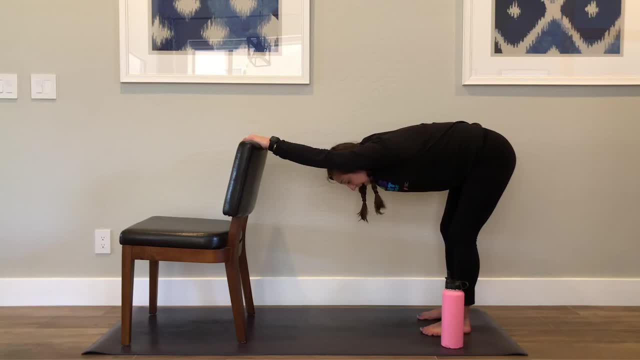 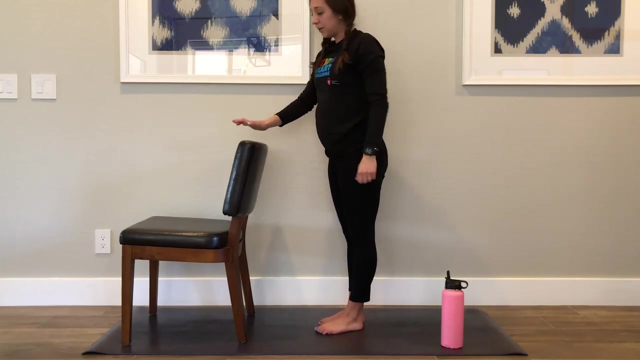 down towards the ground. keep your hands firmly placed here so you should feel that stretch right here in your arms. allow your head to hang heavy. you can sway it side to side, up and down. let that feel really good, great job. now let's go ahead and stand up next. what we're going to do is we are going to place.